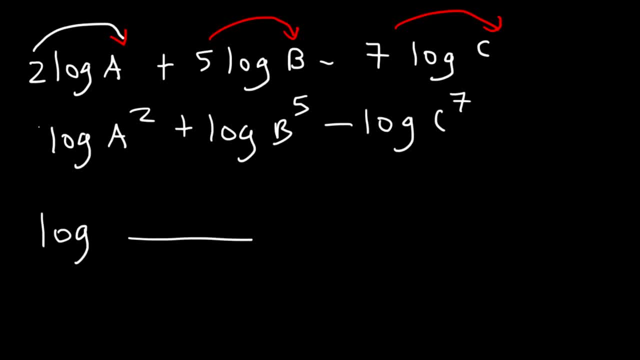 Now we can write a single log. A and B both have a positive sign in front, so they're going to be on top. A squared B to the 5th. C has a negative sign in front of it, so C to the 7th is going to be on the bottom. 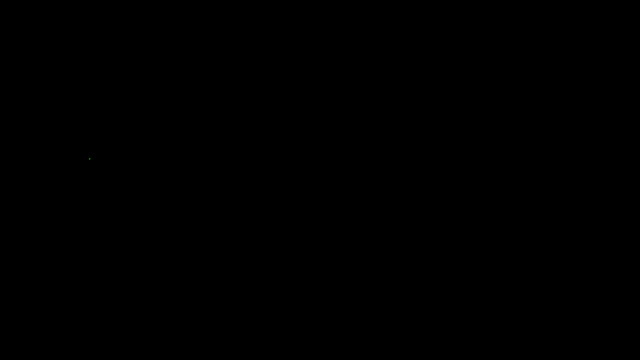 Therefore this is the answer. Try this: one: One third log A minus two thirds Log B, plus one fourth log C minus 4 over 5 log D. So first let's move all of the coefficients to the exponent position. So this is equal to log A raised to the one third minus log B. 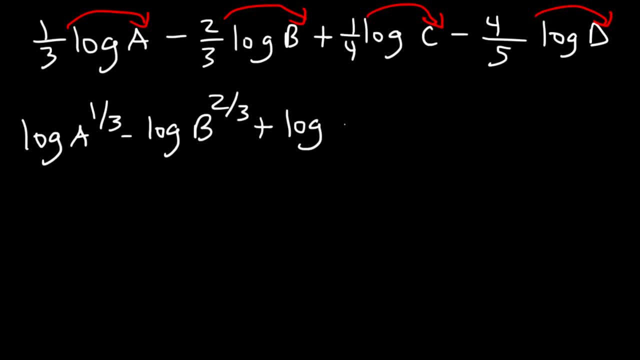 To the two thirds, plus log C to the one fourth, minus log D to the four fifths. And now let's write it as a single log, So A and C both have a positive sign. So it's going to be A to the one third, C to the one fourth on top. 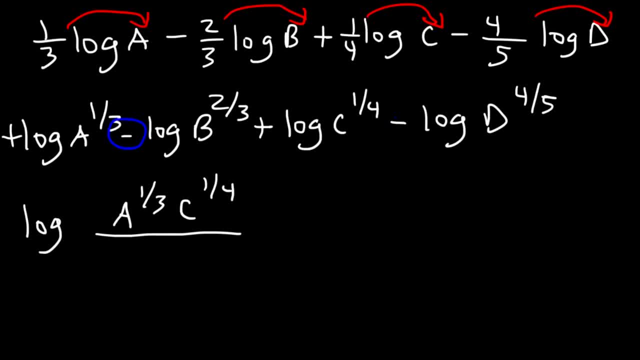 Now B and D both contain a negative sign in front of the log, So they're going to go on the bottom, B to the two thirds and then D to the four fifths. So you can leave your answer like this or you can convert it back into radical form. 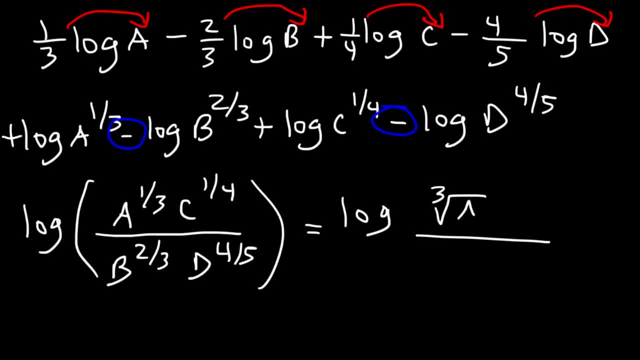 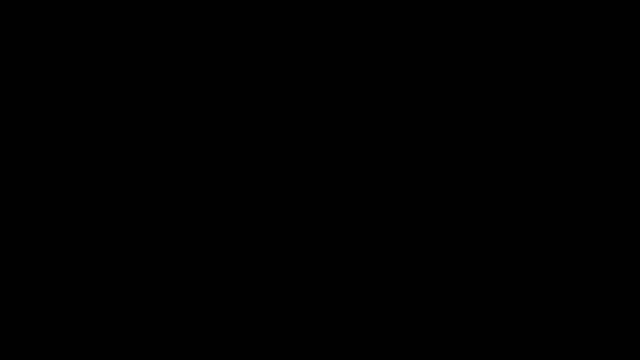 So you can write it like this as well: The cube root of A times the fourth root of C, divided by the cube root of B, squared times the fifth root of D to the fourth. So that's the other root. You can write it like this: 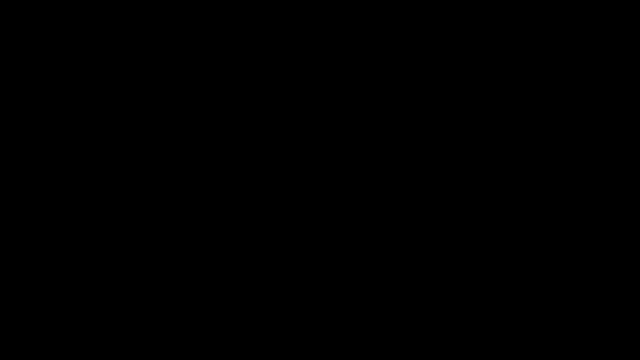 So this is going to be: C equals 4 over 5, log C plus 5.. So you can leave your answer like this. So you can leave your answer like this, And then you can write the rest of the number of your numbers. And the number of rows. So that's the question, And then you can write the rest of your number of rows. So your answer is going to be C over 2.. Like this, Just this, And you have to see what's going on when you write these. So this is going to be C over 2..